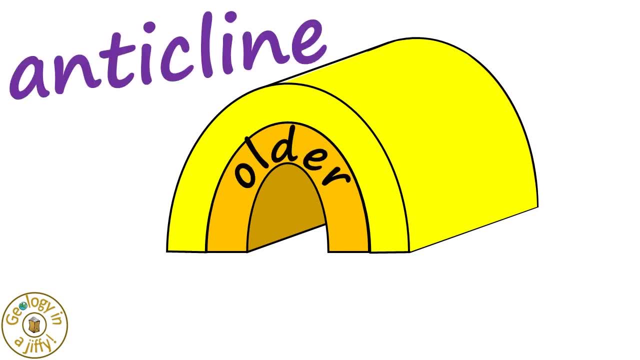 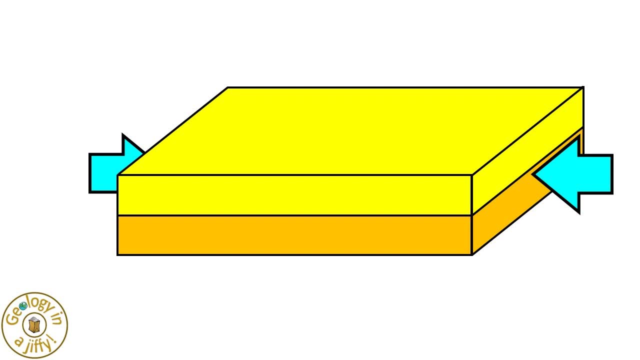 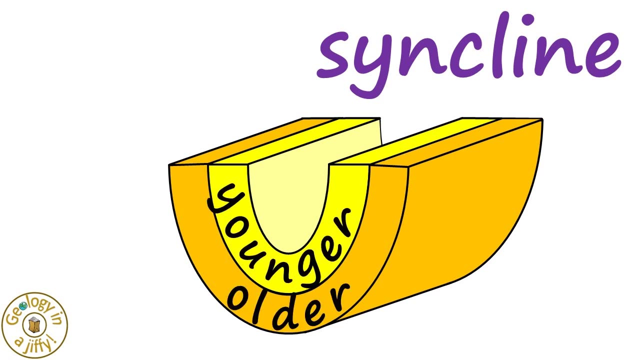 then an anticline forms, with the older layers in the core of the fold surrounded by the younger layers, to the outside of the fold. Alternatively, if we compress the same flat layers but they bend downward, then a synclined forms, with the younger layers in the core of the fold, surrounded by the older. 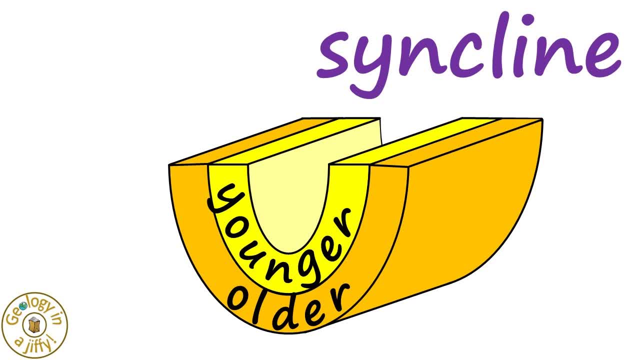 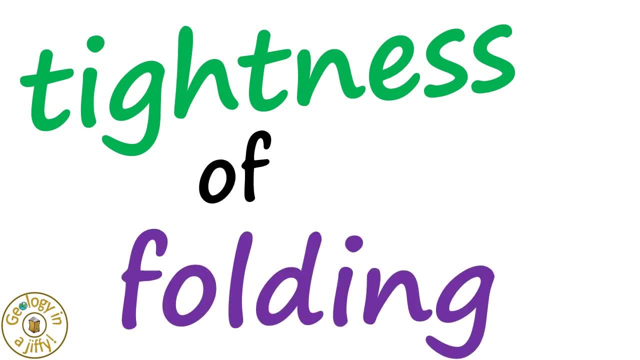 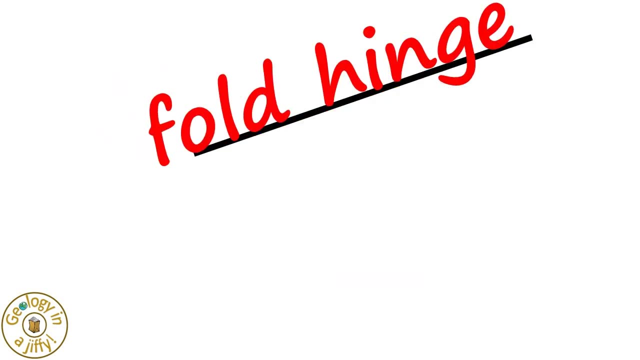 layers to the outside of the fold. Look at the differences. We can study the tightness of the folding too, with three basic types which we measure using a relation of the limbs to the fold. hinge: If the limbs dip gently away from the hinge, then the fold 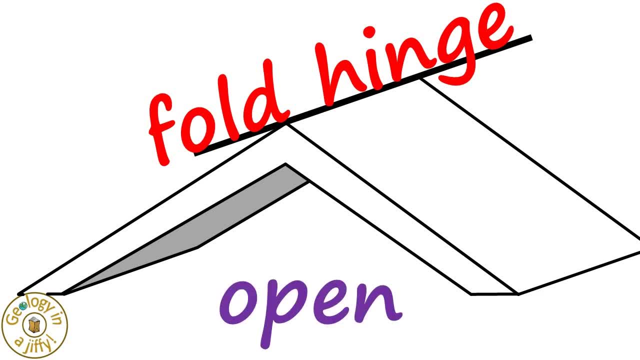 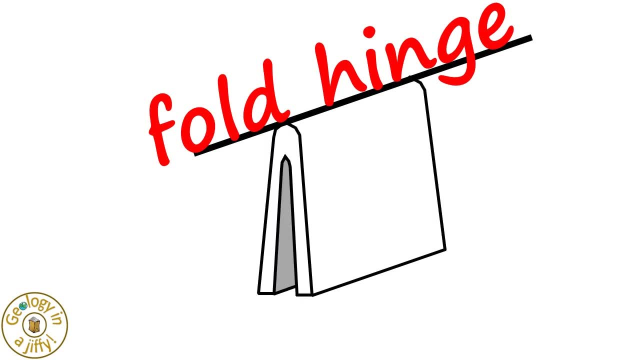 is open. A fold with limbs that are closer together and dipping steeply is said to be tight, And a fold with near parallel limbs is said to be isoclinal. When we compare the fold hinge in relation to the horizontal ground surface, 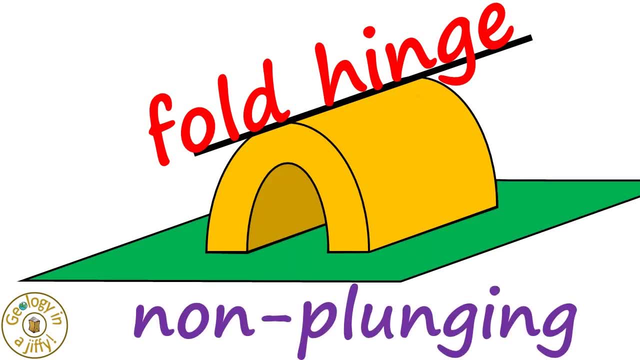 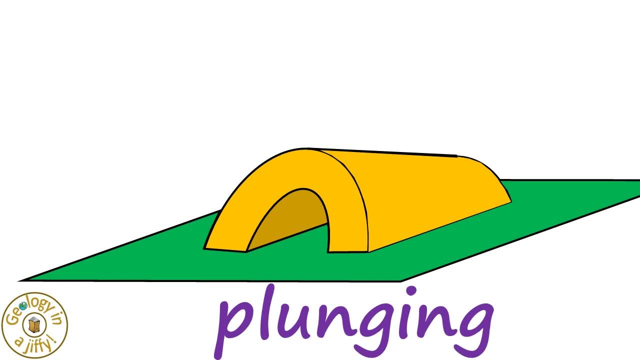 if the fold hinge is parallel to the ground, we say the fold is non-plunging. If the fold hinge is not parallel to the ground, we say the fold is plunging, As this seaward plunging anticline demonstrates. in Cornwall, England, the hinge line dipping away from the land angled down. 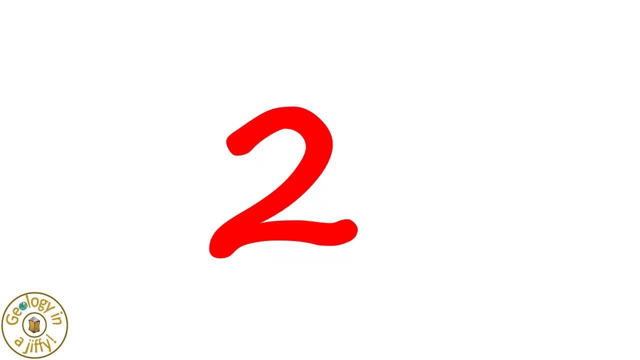 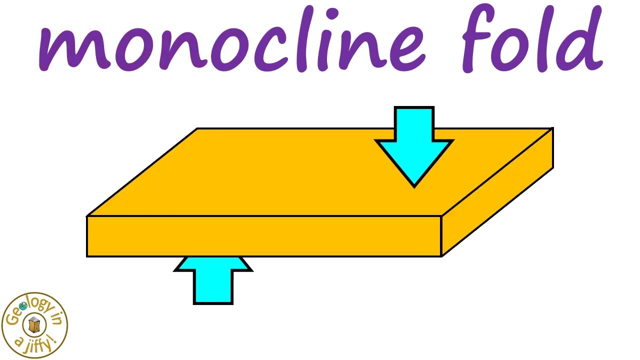 towards the sea. We know the two basic forms of folds are anticlines and synclines, but there are other types of folds. One is a monocline fold, the term mono meaning one. A monocline fold forms due to opposing pressures, forming a fold where both limbs are parallel but offset to each other. 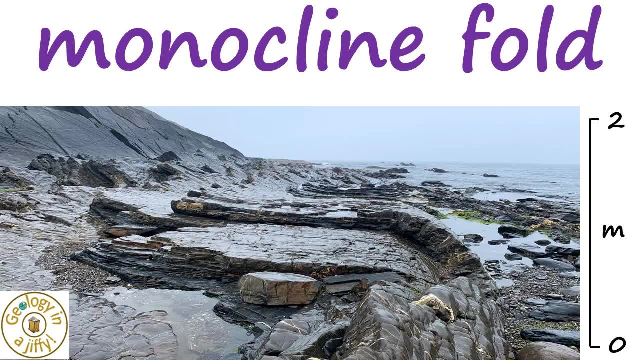 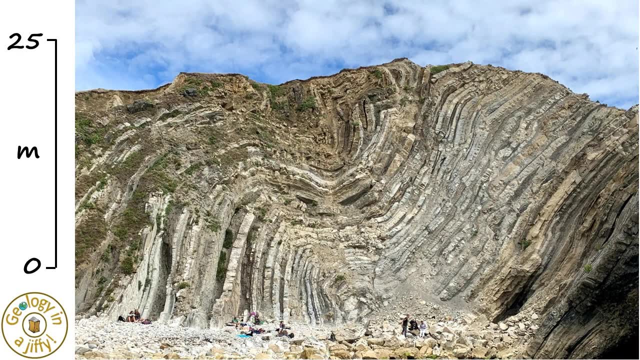 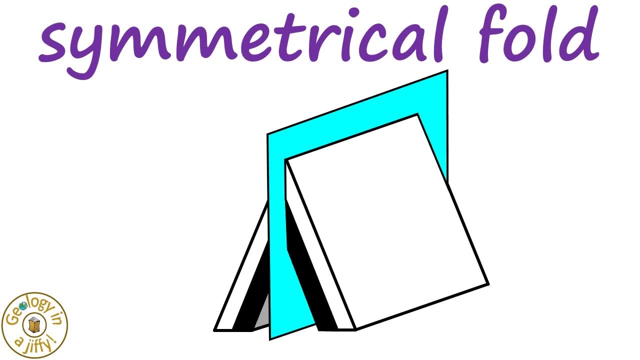 the limbs being horizontal or near horizontal. As seen in the east folded Carboniferous Age Strata in Cornwall, England, and in the Jurassic Age strata of the famous stair hole in Southern England, A symmetrical fold has a vertical axial plane, the limbs being equidistant from the 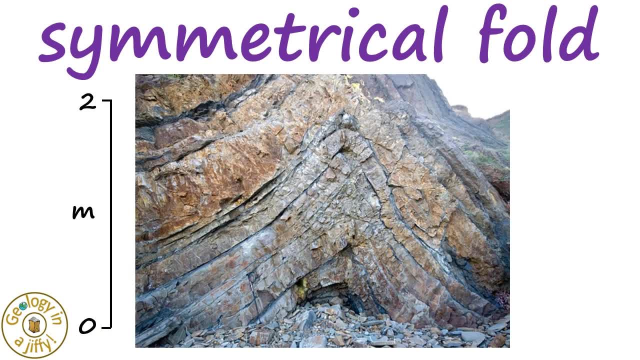 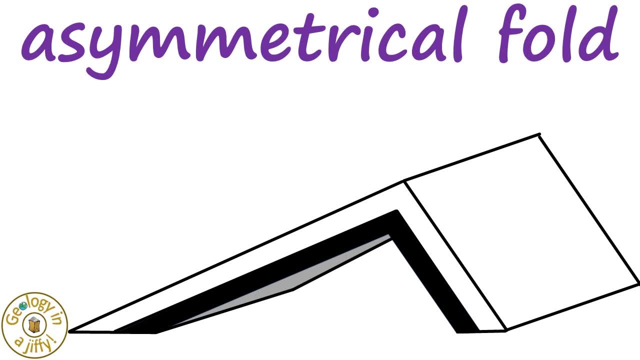 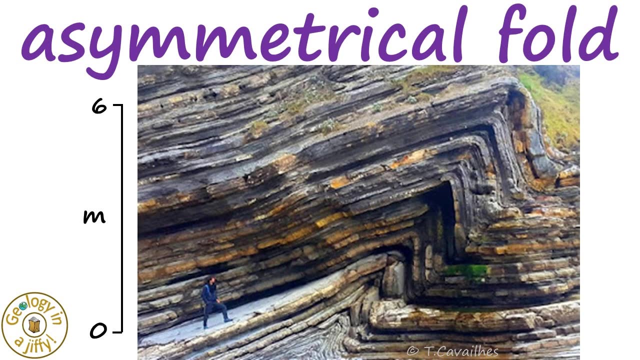 axial plane as demonstrated by the east folded strata in south west England, and a symmetrical fold is one in which the axial plane is inclined, making the limbs dip at different angles, As seen here in folded limestones and mudstones in southwest France.